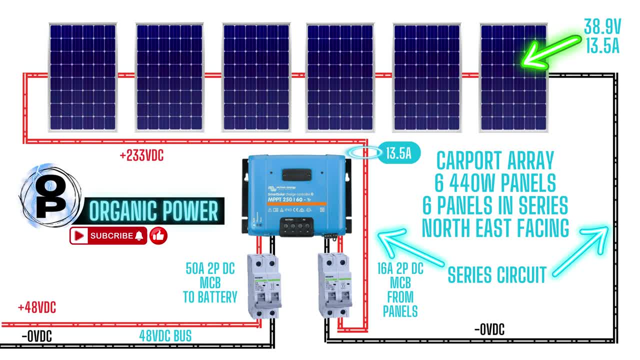 2 pole DC MCB From that circuit breaker. it then flows into the 25060 where it's converted from 233 volts down to 48 volts. It flows then through the 50 amp 2 pole DC MCB Back to the 48 volt battery bus, I thought. 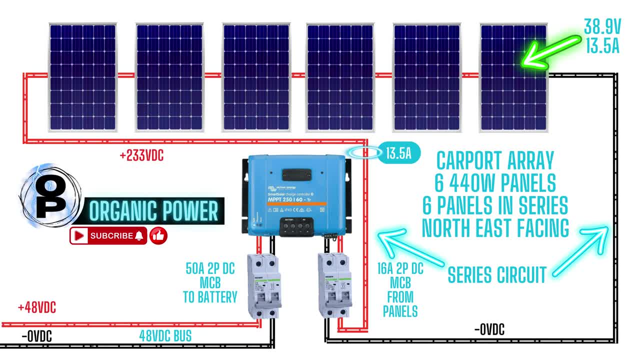 I'd give these bifacial panels a try. There's a great position up there. They're on brackets and they receive a little bit of afternoon sun. It's northeast facing, So collect a fair bit of energy all morning Right up till the 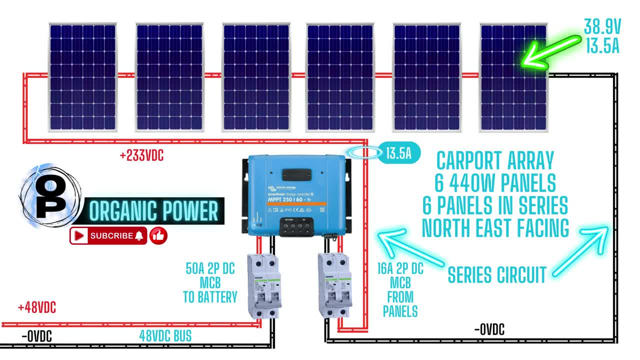 end of the day, And then they even get a little bit reflecting back off the top of the carport into the back of the panel. They provide more power than is actually specified on the panels. This array is a series circuit, So the voltage multiplies as you add more panels, But the current remains constant. 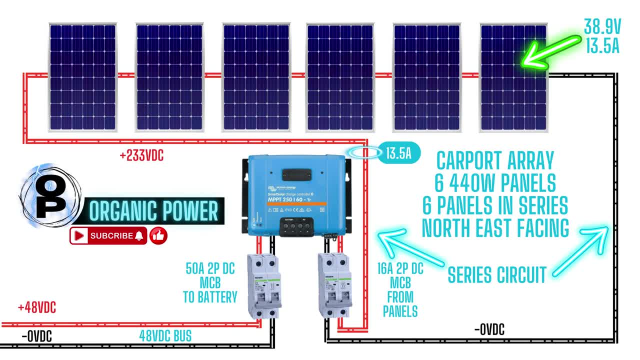 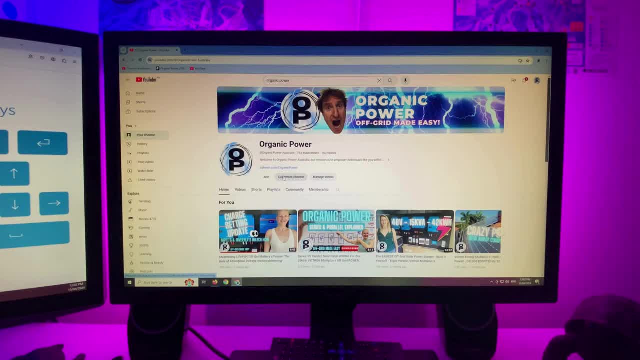 I'll take you out to the carport now and have a look at the array and see how it's connected into the system. While you're here, give us a like, Hit the subscribe button. This way, you can support the channel. Keep the content rolling. This really helps us out. You can. 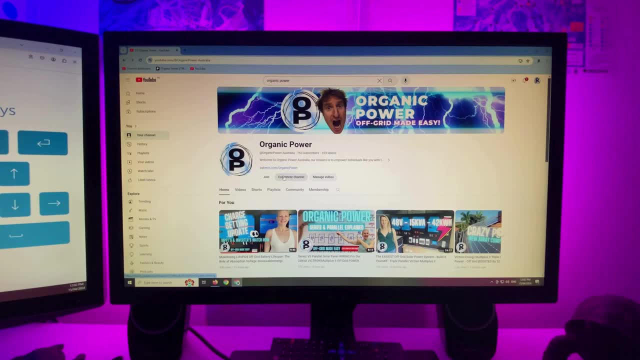 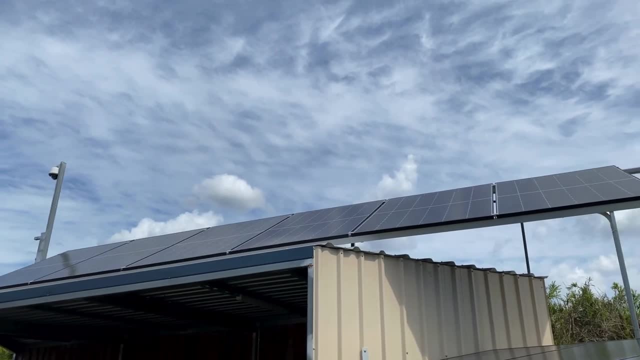 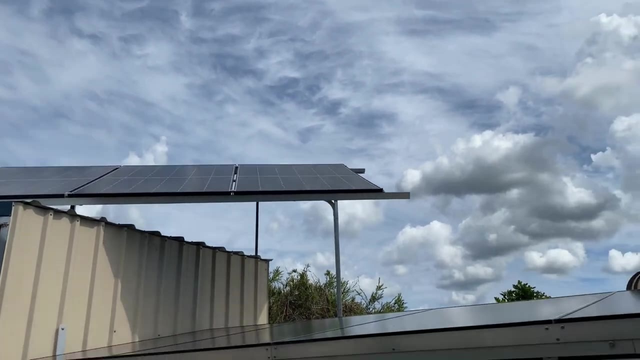 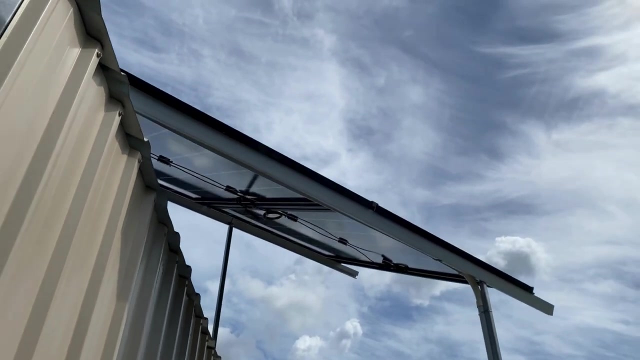 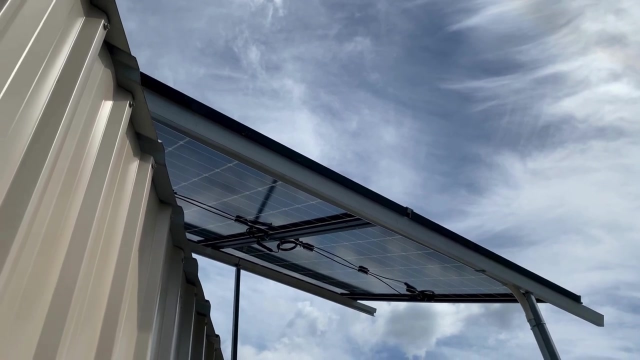 also join the channel and become a member. Have access to all the members only videos On top of the carport. here are the six bifacial panels, 440 watts each, in a series string. You can see on the back of the panel. there It's open to the sun, There's no white. 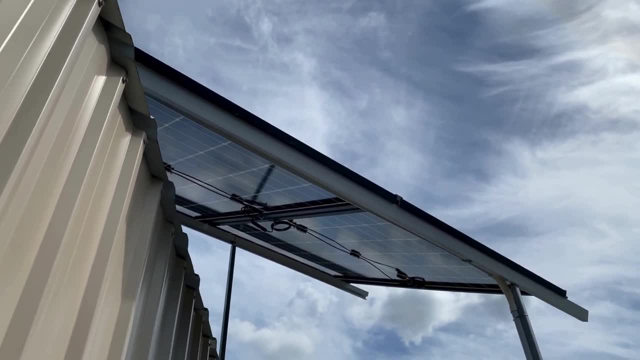 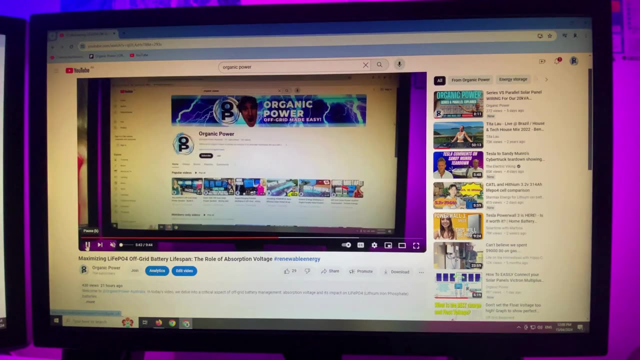 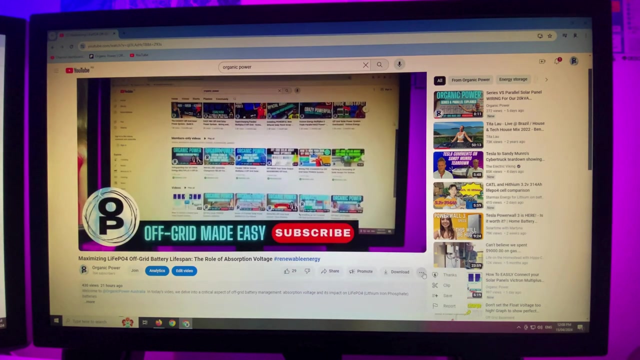 lamination. I'll take you inside the shed now. We'll show you where it's connected into the system. I hope you're all enjoying the content on the channel. Another way to support us is to give us a super thanks. Click the link Now you can. 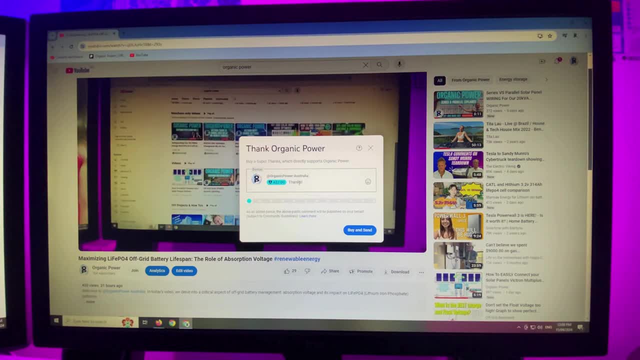 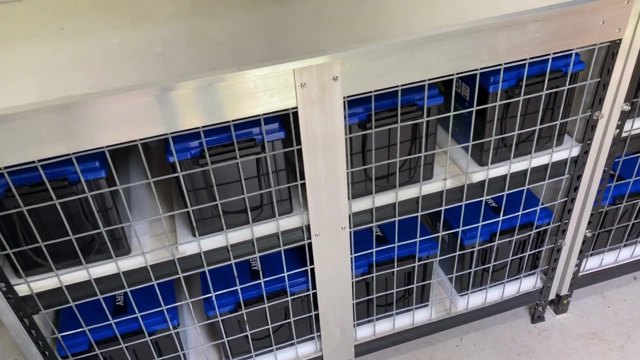 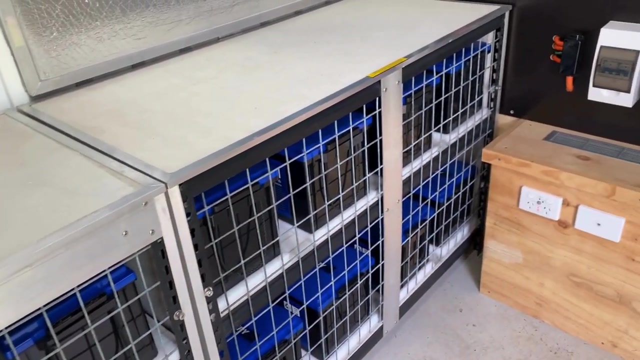 thank us for the work we've been doing, Bringing you all the updates. We can continue to bring you more in the future. So thanks, guys, for supporting us, Liking and subscribing. Here's our 48 volt battery. So that's the bus that the MPPTs feed into. 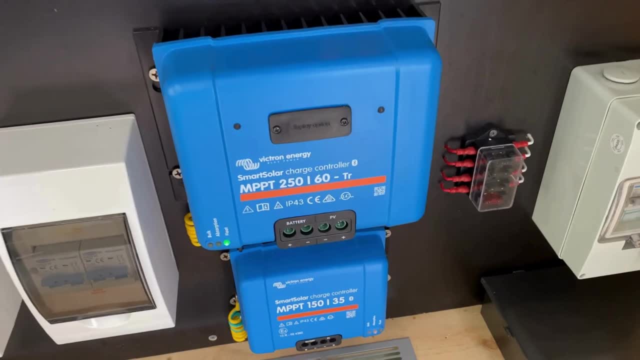 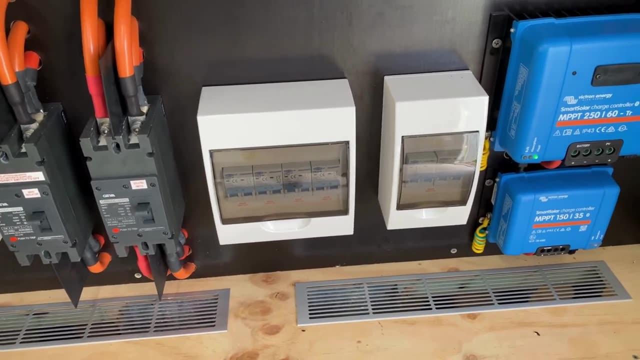 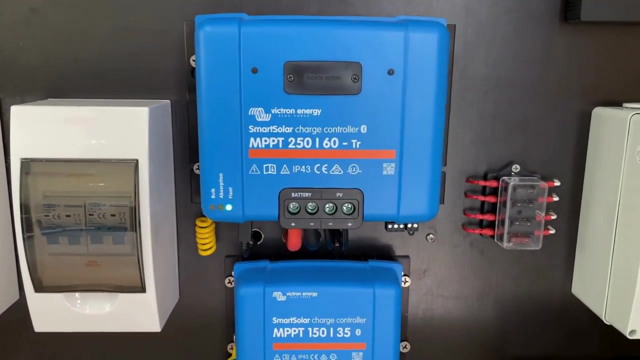 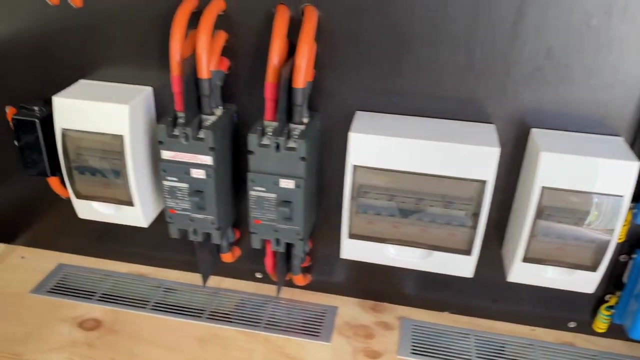 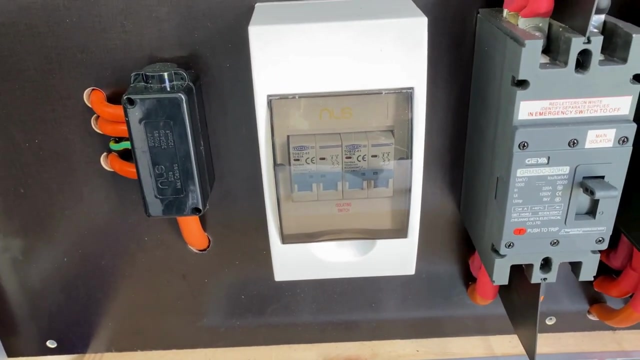 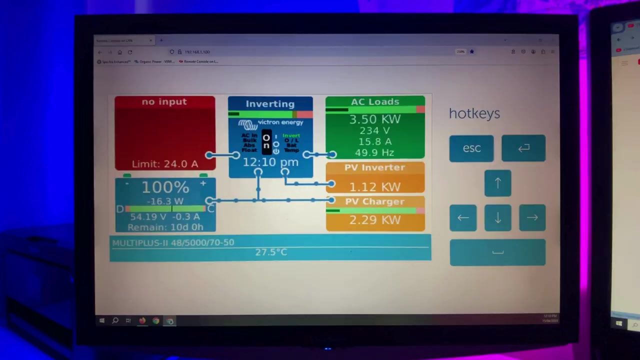 Here's the 250-60.. That's fed from the array by the array breaker And then out of the 250-60 at 48 volts To the battery Through the DC isolator Over to the bus. You may have seen the video I made yesterday About changing the battery charge settings. I went from 56 volts down to 55. And then to 8 volts. This puts a little bit less stress on the batteries, will increase their life, and dropping down to that 55 volt absorption voltage hasn't affected the system whatsoever. We got up to 55, filled the batteries to 100% and went to float. 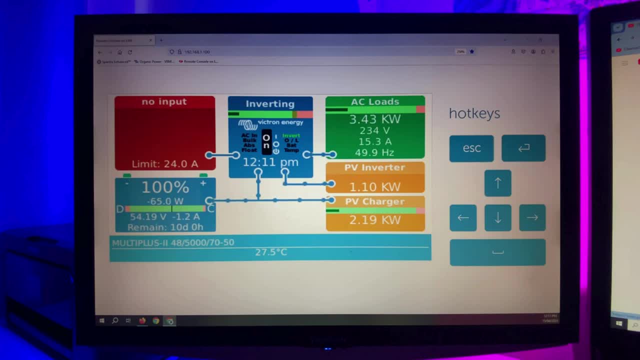 and dropped back to 54.2.. It's a nice sunny autumn day here. The battery was charged by about 10.30. So it's a good outcome. I can now leave that setting at 55 volts. I may as well check the batteries while I'm here. 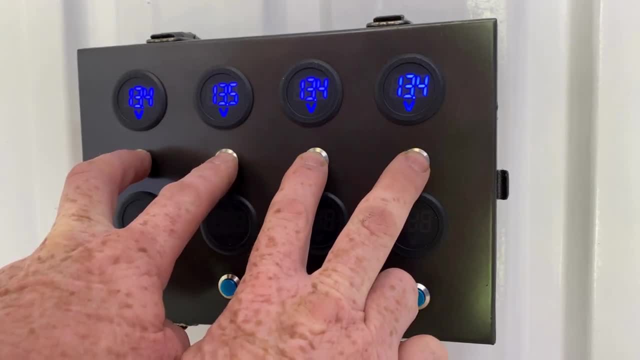 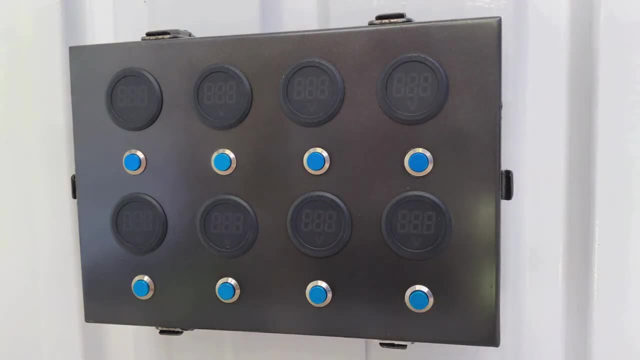 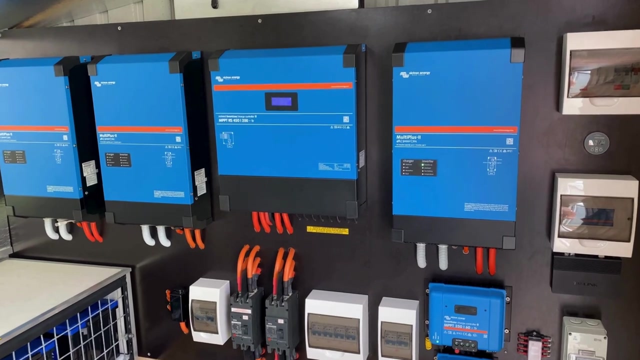 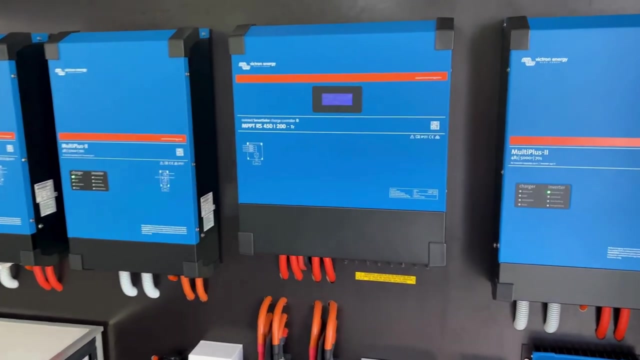 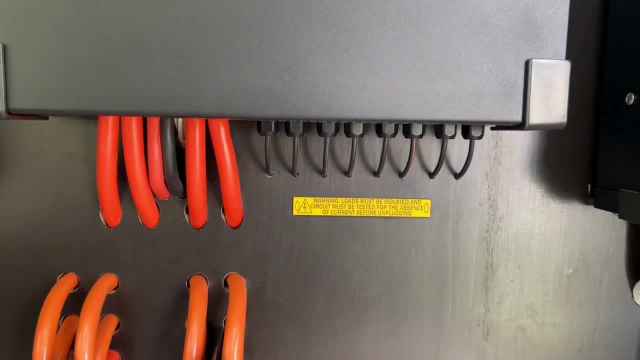 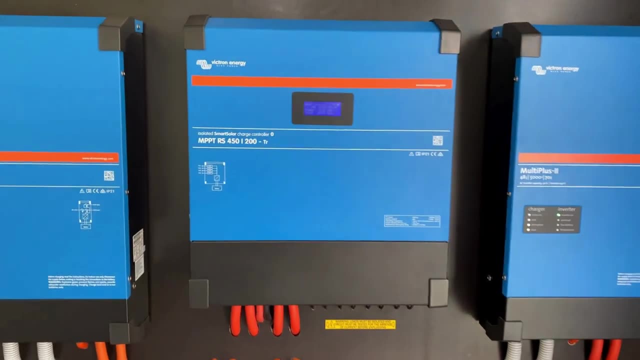 I'm going to connect it to the power supply. I'm going to connect it to the power supply That feeds back to channel 2 of the 450 200.. So stay tuned for that update That'll be out in the next few days. Hit that.